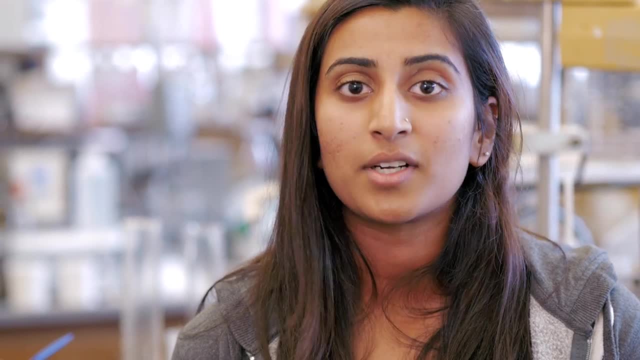 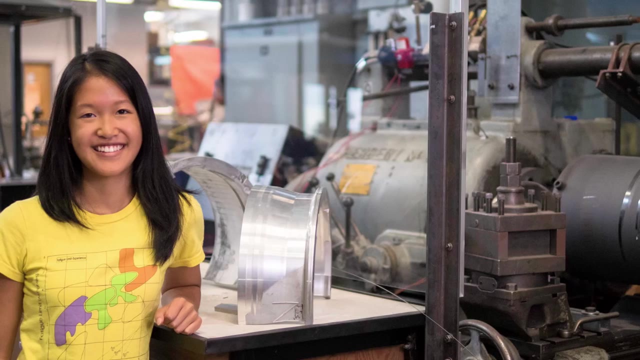 I found myself in the mineral processing stream, which is what I'm currently in. I'm doing my graduate studies in as well. No matter what you get into, you can definitely see materials in every aspect. I'm Vivian Chung. I'm in my fifth year of materials engineering. 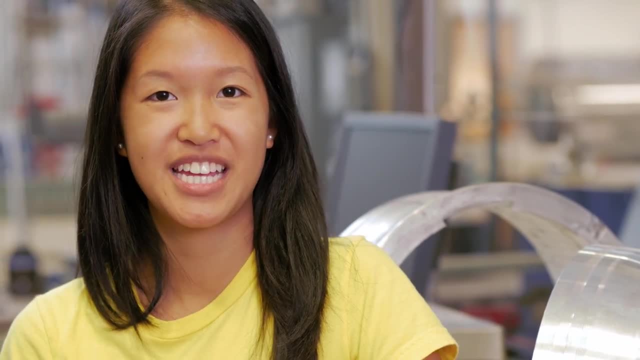 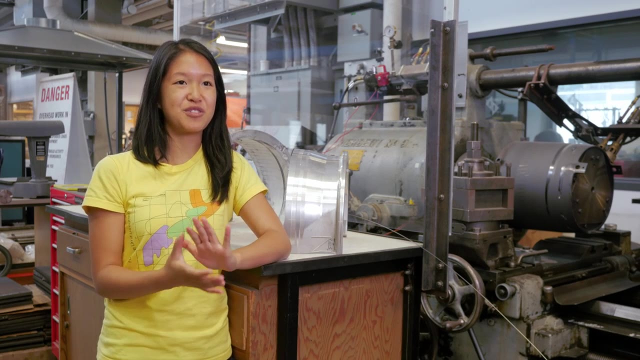 Once I graduate, ideally I would love to get into aerospace manufacturing. So when I first came to materials engineering I didn't know a lot of my friends who had applied to materials engineering as well. So I was kind of I was kind of new, didn't really know a lot of people. 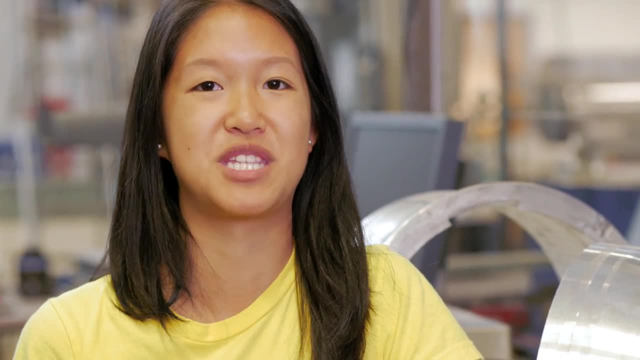 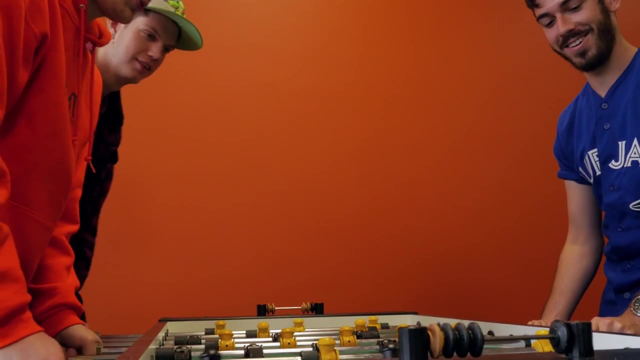 but the small classes really helped with that. You're going to the same class with the same people moving from one to another and you just you get that sense of community. It's a small community in Vancouver, but it's also a small community internationally, So it means that 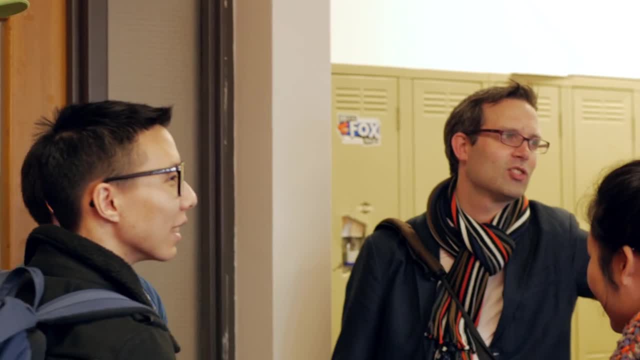 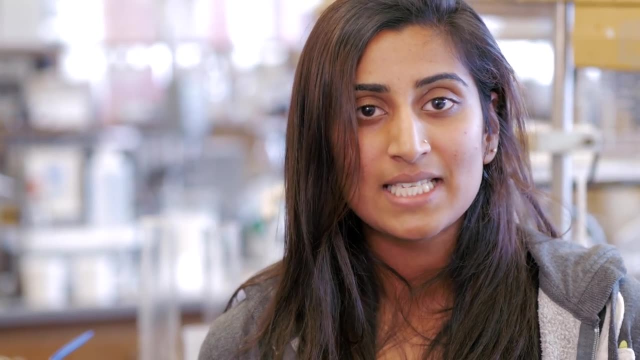 you have connections that come out of the fact that we like to think of ourselves as a kind of family, So people kind of look after one another that way. The researchers and the profs here are amazing at what they do. They have a lot of knowledge and they're world renowned. We have a 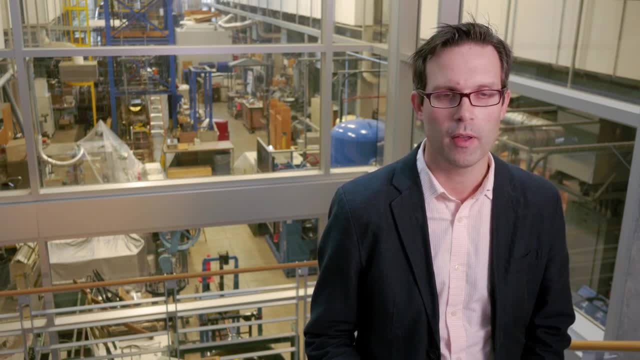 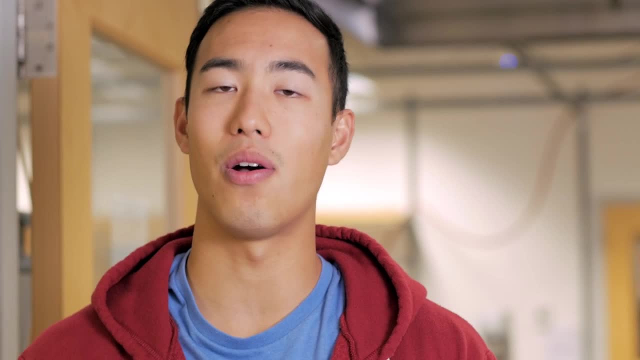 long tradition of working very closely with with industry. We have probably the top group in the industry. We have a lot of experience with the industry. We have lots of experience with the industry. We have a lot of experience with the engineering technology and technology. 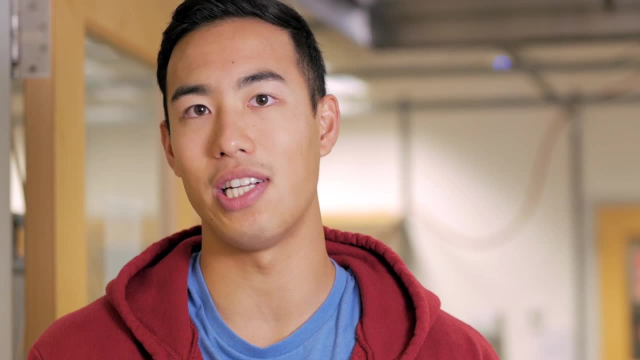 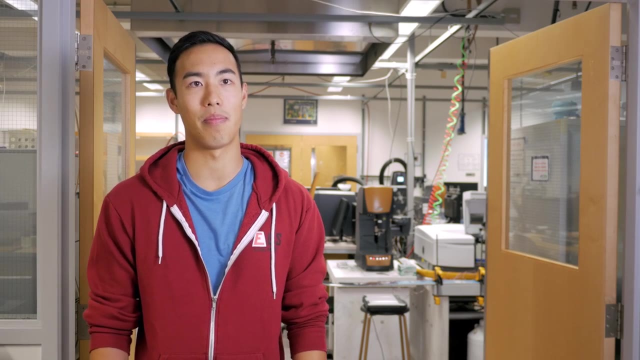 within our department. You get all sorts of support, not only from those professionals who have worked in the field for many years, but also from your peers, because you rely on each other for support and you see each other every day and you know everyone's name. You really get that. 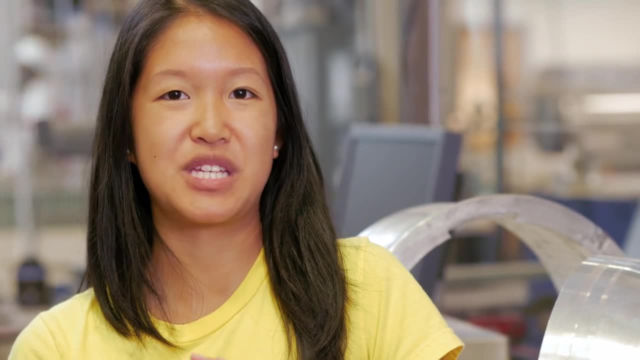 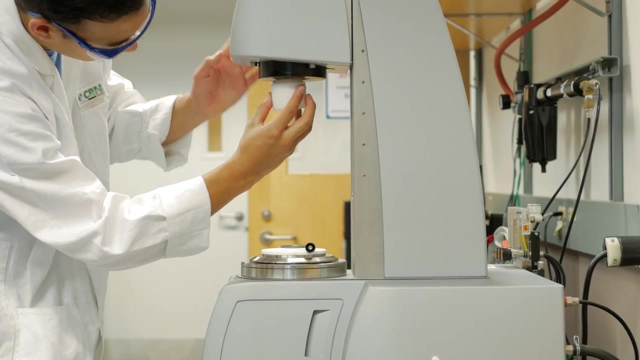 opportunity to build that community within your program. Something that I wish that I had started earlier was just getting involved with everything, So I think it's super important for people to get to a real application. This lab is part of the Composites Research Network. 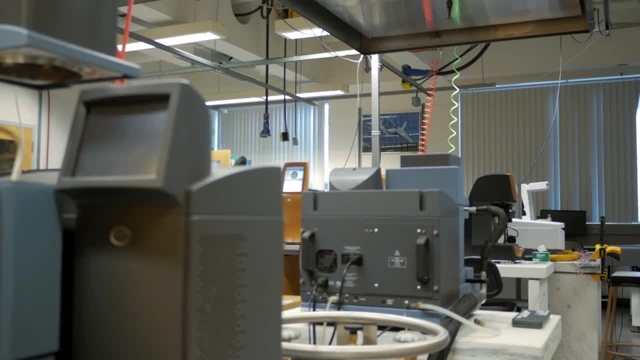 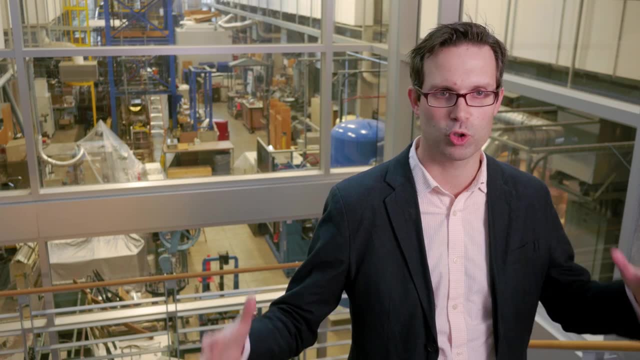 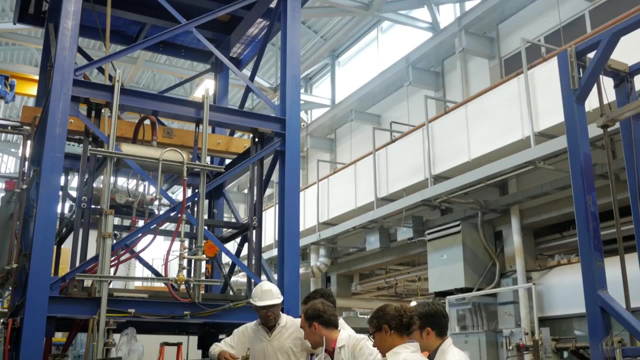 We have research that occurs here by master's students and PhD candidates. We also bring in a lot of projects from industry. The space that we have behind us was specifically designed to house large-scale experimental apparatus, apparatus that is meant to simulate what happens in actual industry.